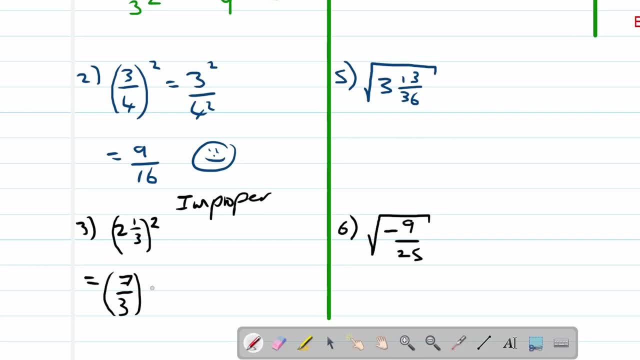 7. So it's 7 over 3 square, Which is 7 square over 3 square, Which is equal to 49 over 9.. Do we have any common factors there? No, we don't. Therefore, we are done. These were the examples. 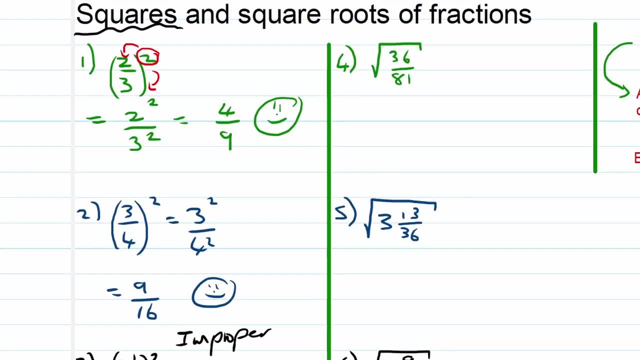 regarding squares specifically. Now let's move over to square roots. Same rules apply. You take the square root of The numerator Over the square root of the denominator. Now we apply it separately. Square root of 36 is equal to 6.. Square root of 81 is equal to 9.. Do we have any common factors here? 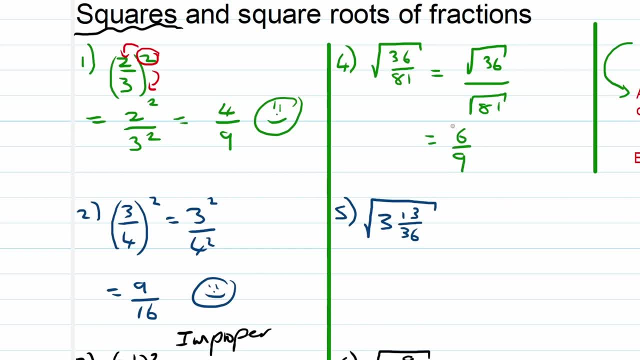 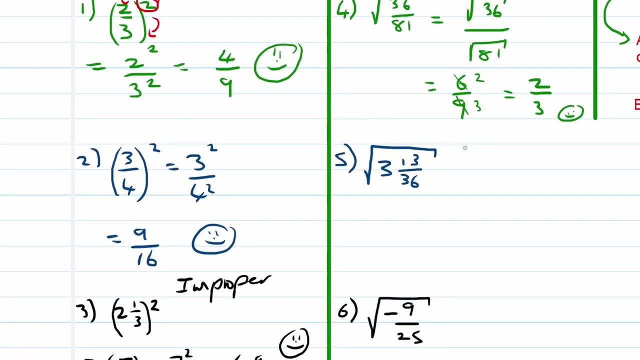 Yes, we do. We've got 3 as a common factor. 3 goes into 6 twice, Into 9 three times. So this will be simplified to 2 over 3.. Let's move over to the following example, Example 5.. And we've got a mixed number yet again. So what's our very first step? 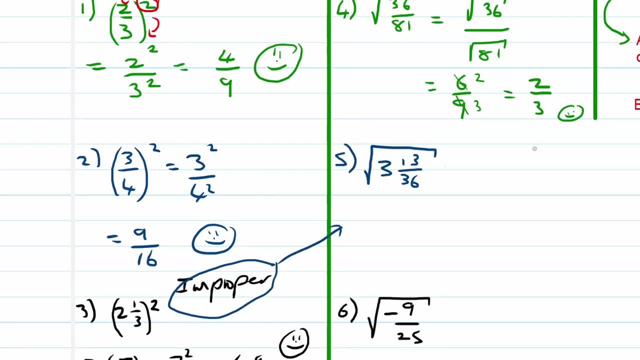 Improper fractions. We have to write it down as an improper fraction, So that means the square root of Now. let's see: 3 times 36 is 108.. 108 plus 30 is 121.. 121 over 36.. 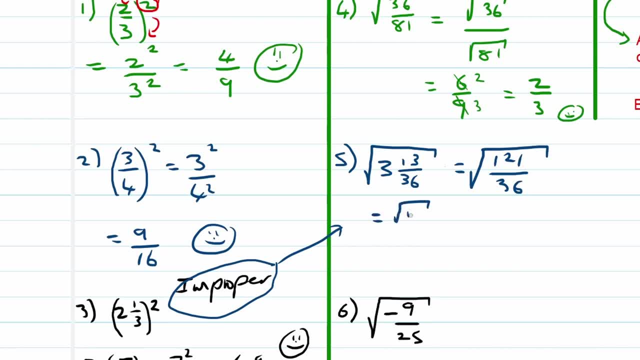 Now we're going to apply the square root at the numerator and denominator Separately, And the square root of 121 is 11.. Square root of 36 is 6.. Do we have any common factors here? No, we don't. Therefore, we are happy and we're done. Let's look at 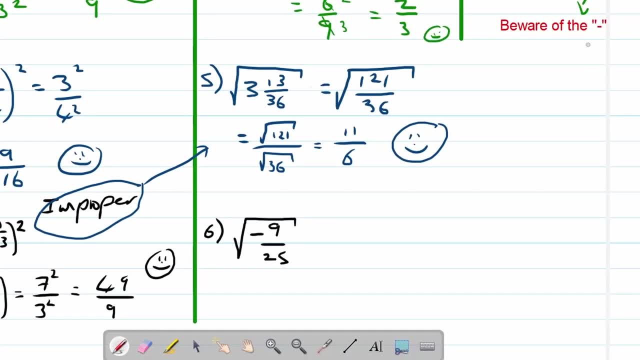 the last example, And this is where we need to be aware: Beware of the negative, Beware of the negative. A negative number underneath the square root is undefined. Therefore, it has no solution, No real solution. Okay, So no solution. Very important, The moment you see a negative underneath the square. 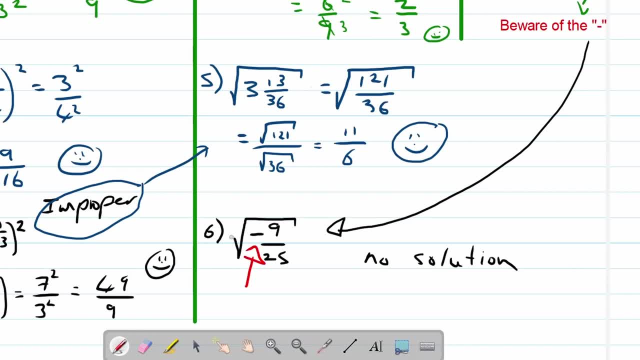 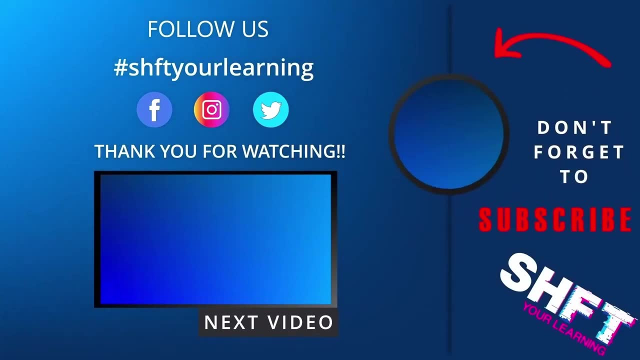 root. This only applies if it's a square root or a fourth root or a sixth root or an eighth root, An even number root, Then this applies. Then we'll have no solution. So enjoy Happy practicing. See you soon. Subtitles by the Amaraorg community.